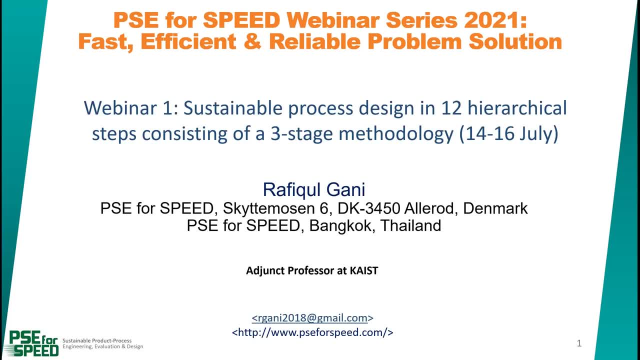 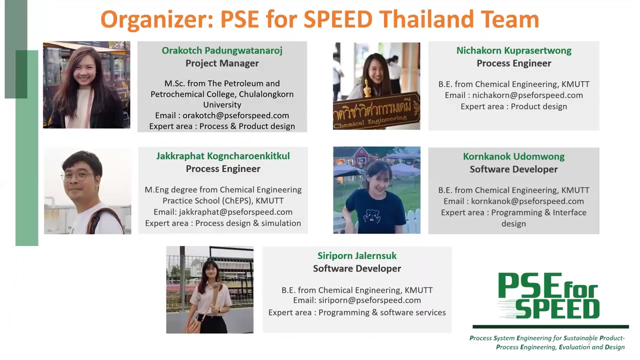 Sustainable process design in 12 hierarchical steps consisting of a three-stage methodology. I'm Rafi Kulgani, I'm the founder of PSE4Speed and also our headquarter is in Thailand, and let me introduce you to the members of the Thai office. starting with, I will just say the first names. 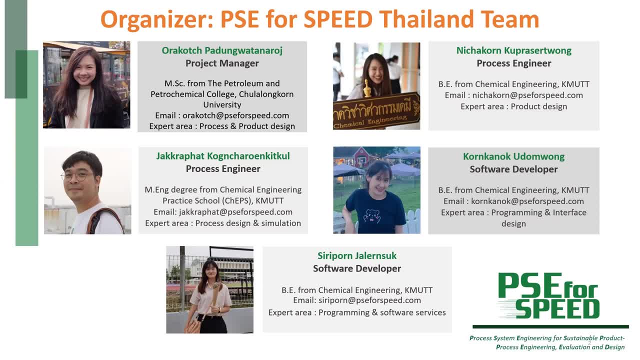 Urakotch, who is the project manager of the office in Thailand, then Nichakorn, who is a process engineer, expertise in product engineering, then Chakrapath, also a process engineer, and his expertise is in process engineering. and then Konkarnok is a software developer. 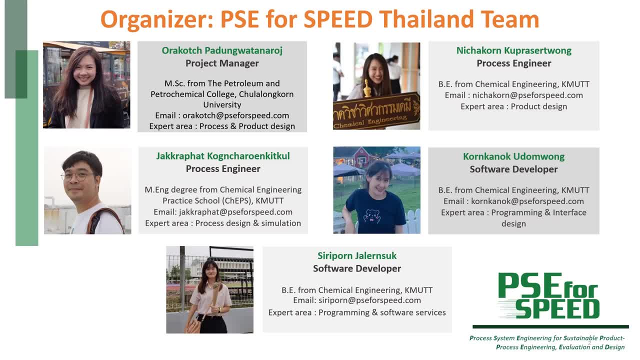 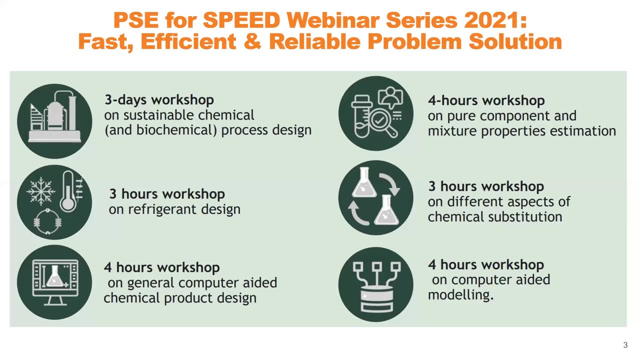 and also Siripon, a software developer. So thanks to all of you for getting this initiative started. As you have seen from the brochure, there are six webinars. The first one is over three days, then there are five others which are one day webinars. 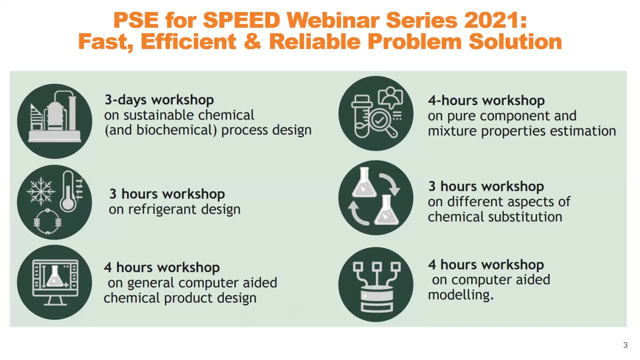 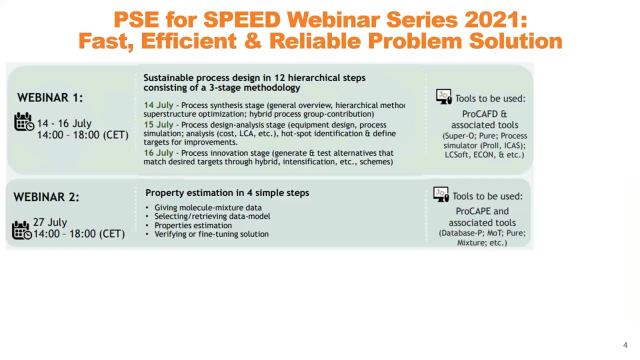 So webinar one and two are on this month after the. the set of three webinars today, tomorrow and the day after related to process sustainable process design in three stages. then we have the property estimation in four simple steps on 27th of July. Then webinar two is about 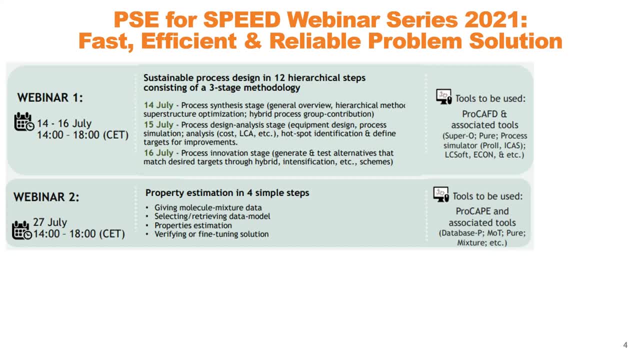 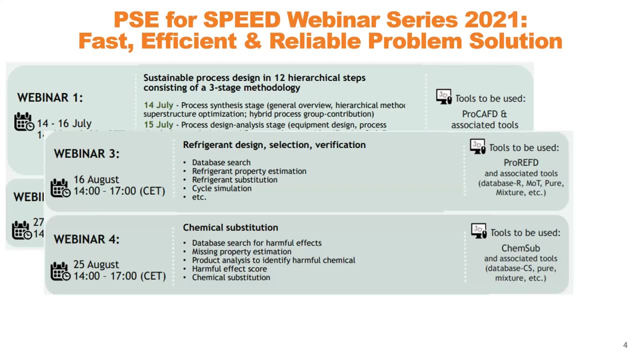 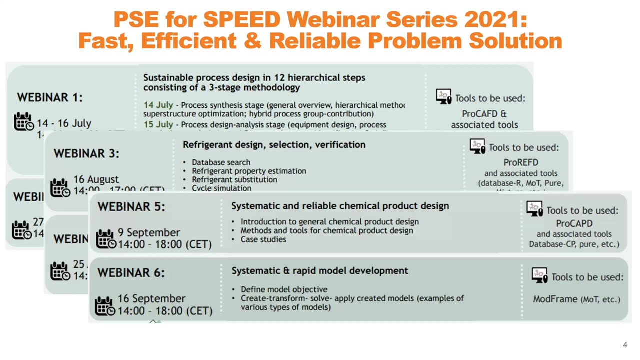 the management. Thank you. Webinar three is about refrigerant design selection verification on 16th August. Webinar four is on 25th August on chemical substitution. Webinar five is systematic and reliable chemical product design. And the final one, webinar six, is systematic and rapid model development. 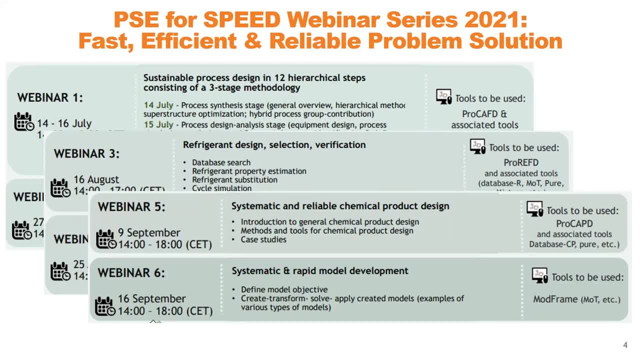 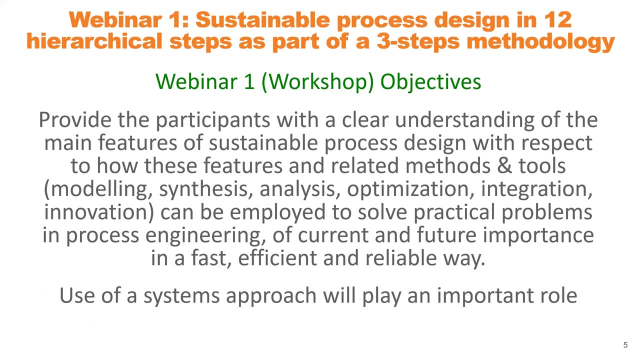 In all of these webinars we also have an invited guest lecturer, Which you can see in the brochure. So let me start with the objective of today's webinar. Not today's, but the series one, two, three of today, tomorrow, tomorrow and day after webinar. 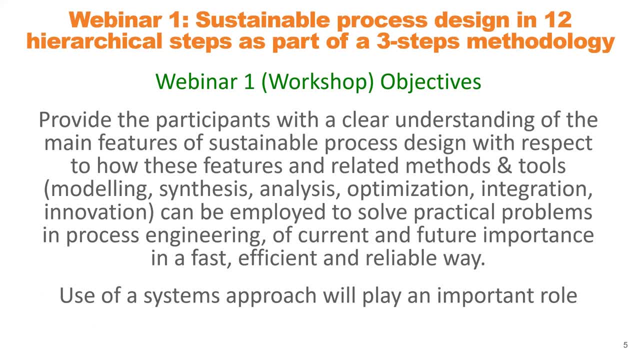 The objective is to provide the participants with a clear understanding of the main features of sustainable process design With respect to how these features and related methods and tools- Modeling, synthesis, analysis, optimization, Integration, innovation- can be employed to solve practical problems in process engineering of current and future importance in a fast, efficient and reliable way. 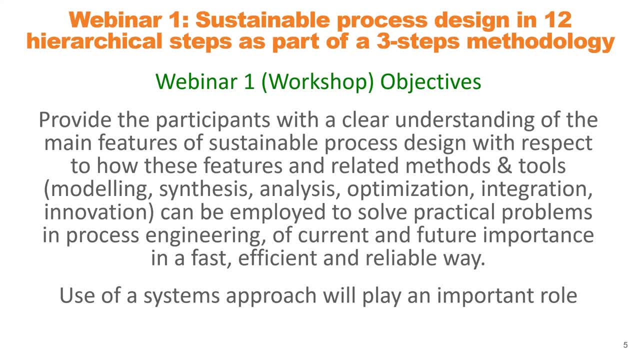 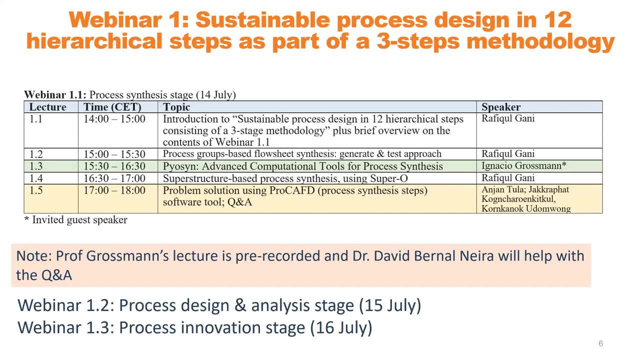 Use of a systems approach will play an important role. More specifically, today's webinar consists of five sessions. The first one is a lecture that I'm giving, Where I will introduce The concept of sustainable process design in 12 steps, in three method, three-stage methodology. 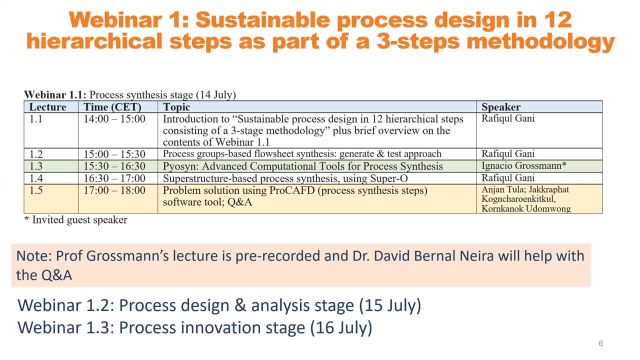 After that I will also give a brief overview on one of the synthesis methods, That is, the group contribution-based generate and test. Then Professor Ignacio Grossman will give a recorded lecture. It's too early for him in California now, So he sent us a specially recorded lecture and that will be on biocene: advanced computational tools for process synthesis. 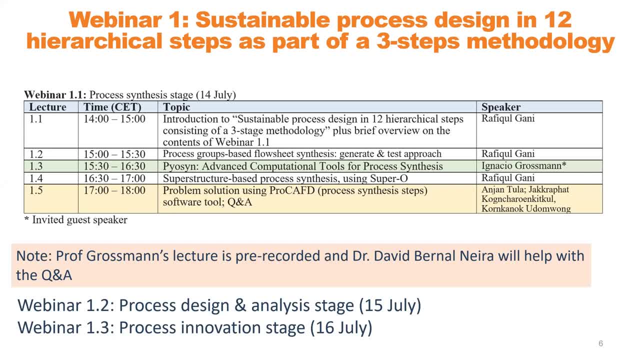 After that, I will again give a short presentation on another way of doing superstructure-based process synthesis using Super-O. And finally, the last hour will be on problem-solving. And finally, the last hour will be on problem-solving Through our special software, ProCFD, highlighting only the steps of process synthesis. 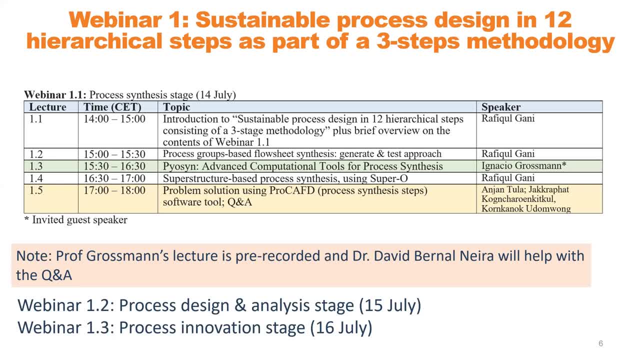 For each of those, each of the sessions, there will be time at the end for question-answer For Professor Grossman's lecture. Dr David Bernal-Naira, who is a former PhD student of Professor Grossman, has kindly agreed to join the discussion and answer any questions for me. 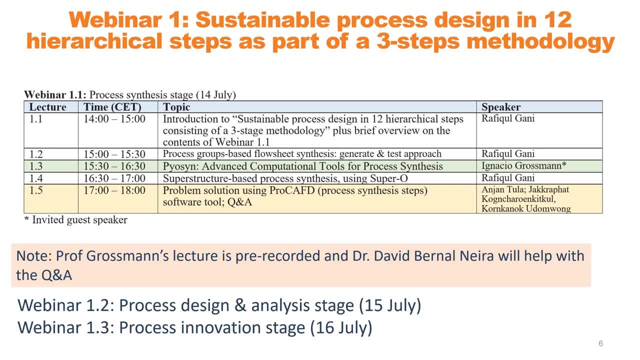 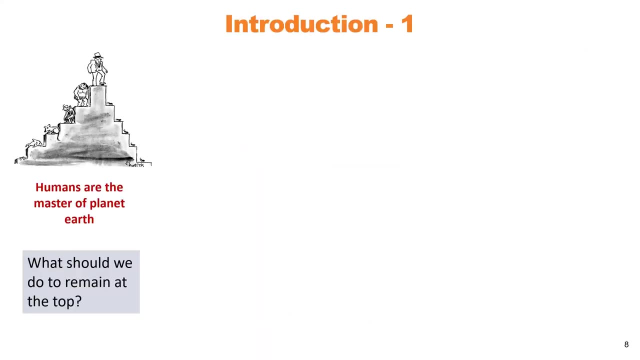 So thank you very much. In the series tomorrow and day after, we will have process design analysis stage and process innovation stage. So let me start with the big picture. We know that we humans are the master of planet Earth, but the question is what we need to do to remain at the top. 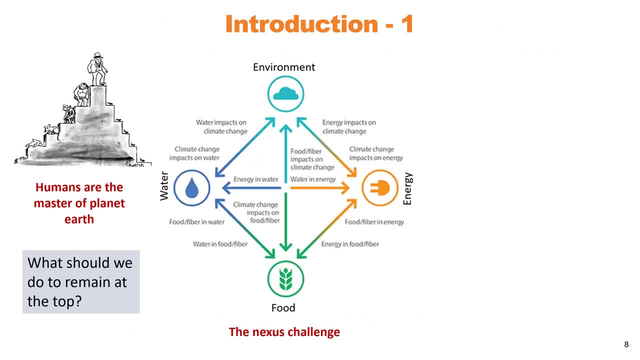 And one of the challenges facing us is the challenge of water, energy, Food, environment and their interactions. How do we address those challenges? That is the sustainable solution we are looking for. So the workshop highlights the relations of energy, water, food with environment and associated challenges to find sustainable solutions. 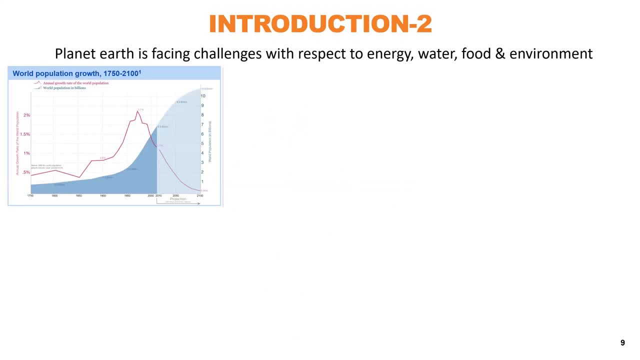 And why is this a problem? Let us look at the data. The figure you see- The blue one- is the population growth on Earth and in the next- by 2050, we may reach around 10 billion people. So what does 10 billion people mean? 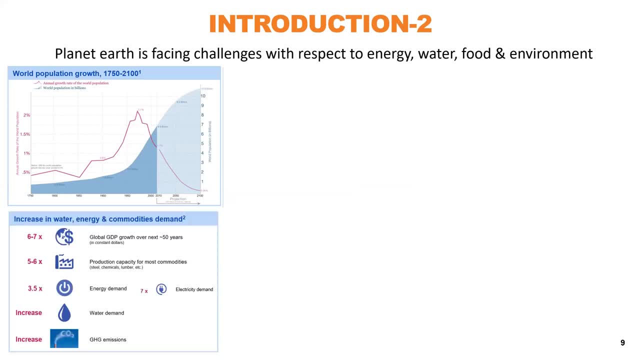 Which means also that within the 2050, we will need six to seven times increase in the global GDP. That will require Five to six times the increase in the production capacity for most commodities, And all of these will require more energy demand, more electricity demand, more water demand and all the activities will increase the greenhouse gas emissions. 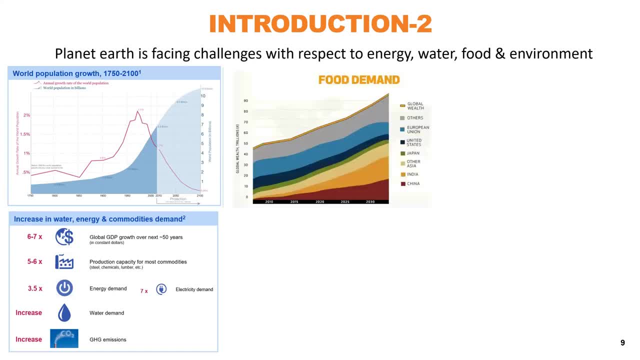 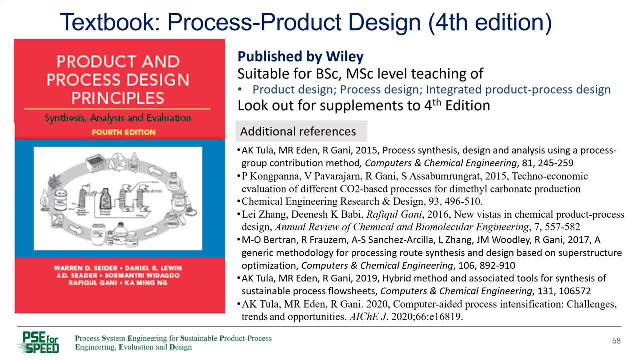 If we look at the energy, the demand for energy is increasing. The properties are classified, which actually will be presented in the next lecture. There are different kinds of properties. One property is related to the environment. If this chemical product is going to somehow go to the environment, 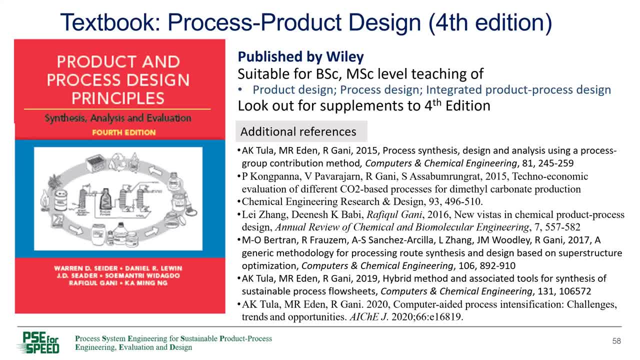 what kind of effects it will have. So environmental properties need to be looked at, then. properties related to the environment, to their stability, their separation, boiling point, melting point, phase equilibria. There's a whole lot of list of properties that are needed, and we will discuss them in the next presentation. 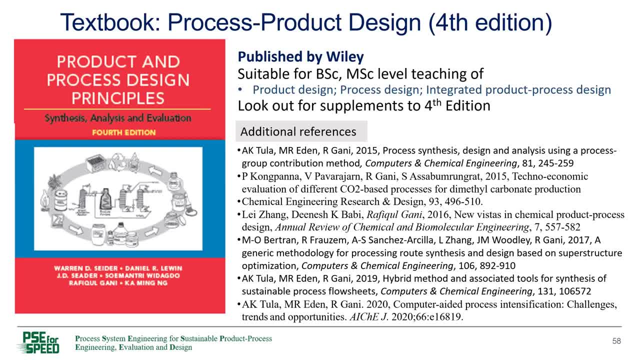 Okay, another question. And another question is: is it possible to do process synthesis for automatic product system in one go, For example, a new promising technology where production of various products from the same feedstock is possible? Yes, definitely, it is possible. We will show with the superstructure optimization. 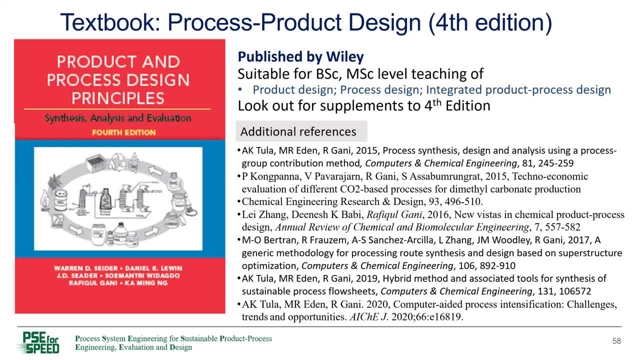 how it is possible. I can see that Lucas has raised hand. Yes, Lucas, you can speak now. Yeah, thank you very much. Thank you for the nice presentation And I wondered in the beginning you showed possible ways to reduce the environmental impact of the chemical. 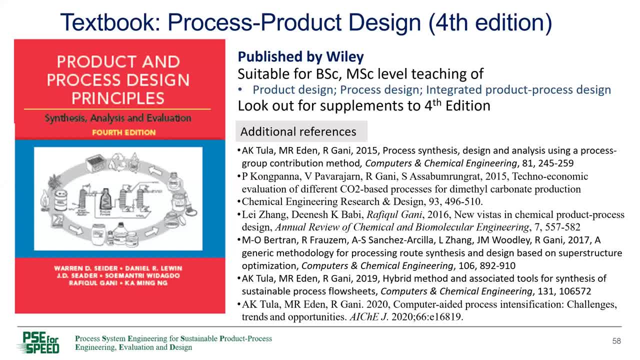 industry in general, And I was wondering where you would put things like renewable, how to say biobanks, Biobank, Yeah, yeah, yeah. So, for example, where do you mean? these products is somehow fossil fuel-based products instead of fossil fuel-based products? 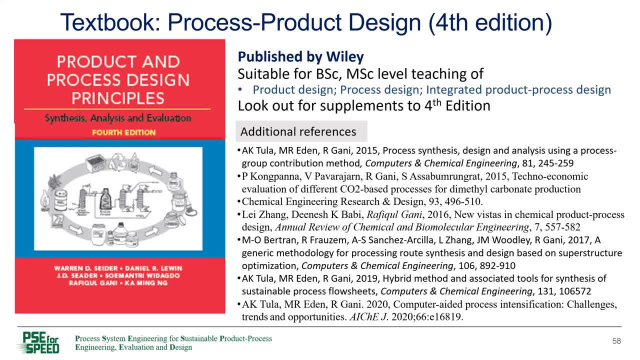 Yes, Actually. I mean, this lecture was just an introduction and only the evolutionary methods, so I didn't highlight any of those things. But in the lectures- remaining lectures today and also tomorrow and day after- you will see that all these questions are answered. 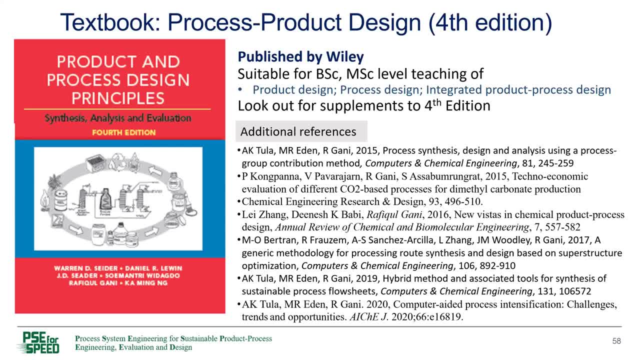 looking for is actually. that's why I mentioned the system boundary, Because within the system boundary, we want to say that we will take a system boundary that includes the power supply, the energy supply, the water supply, the process, the by process, And then we have to make a network of all of these.